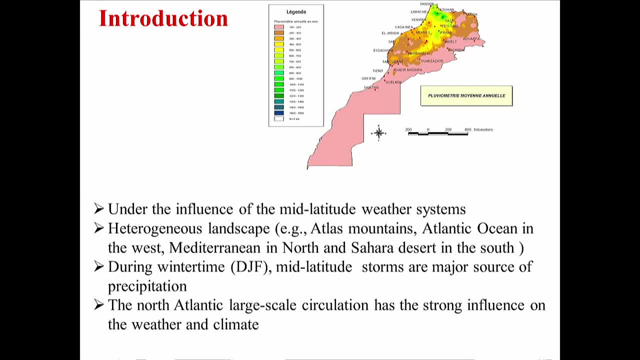 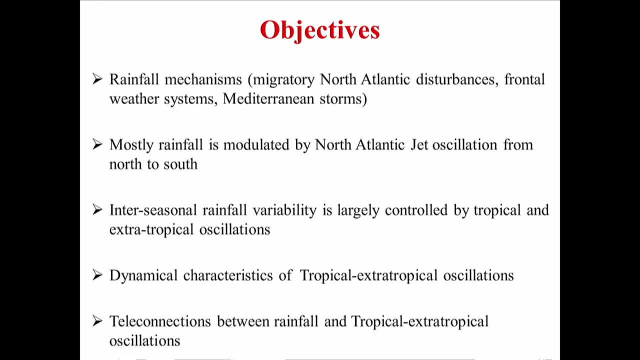 has a strong influence on both the weather and climate. Our objective is to see how this migratory North Atlantic disturbance, frontal systems, mid-rhineland storms and the MGO-NO regime can influence the weather and climate. So we want to see how this migratory MGO-NO regime can influence our rainfall mechanisms and 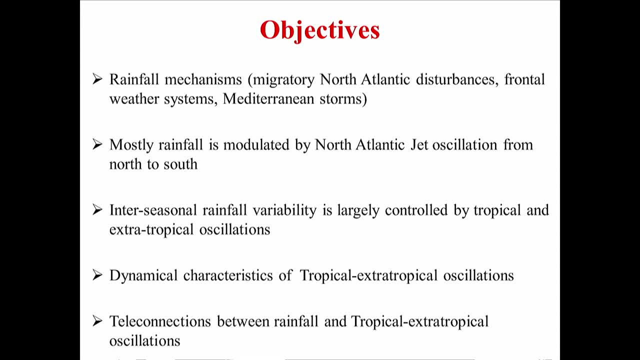 how they are modulated by some large-scale patterns. In fact, most rainfall are modulated by North Atlantic jet oscillation from north to south and there is a kind of seasonal variability which is controlled by this tropical-extra-tropical oscillation. We want to understand how this tropical-extra-tropical 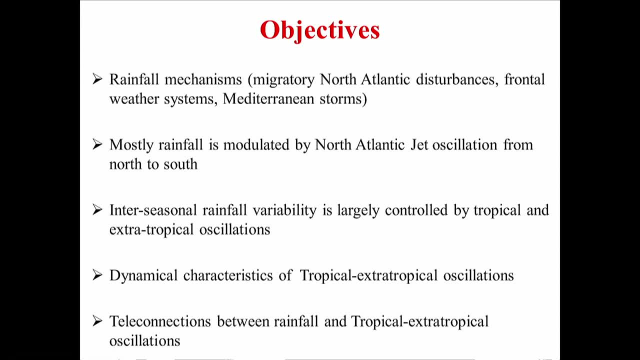 oscillation can affect our rainfall mechanisms and how they are modulated by some large-scale patterns. And we want to see how this tropical-extra-tropical oscillation can impact our rainfall mechanisms and how they are modulated by some large-scale patterns. And the next objective is to see how can we forecast the weather and climate at subsistimal 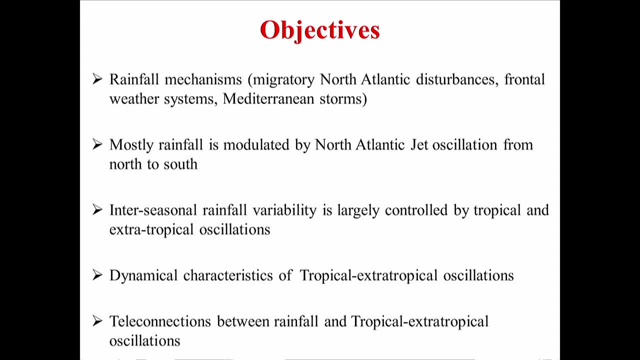 scale, using this connection between rainfall and tropical-extra-tropical oscillation. And finally, we will see how the weather and climate can affect our atmospheric dynamics over Morocco. And finally, we will see how the weather and climate can affect our atmospheric dynamics. 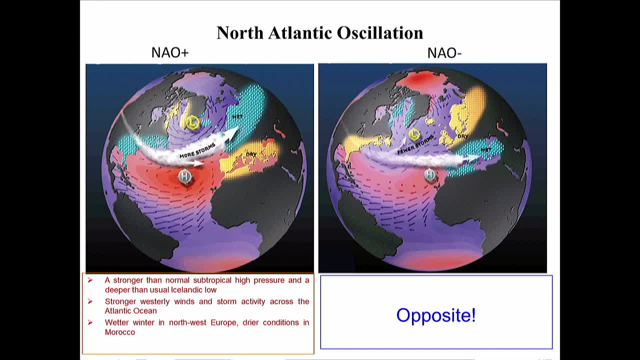 over Morocco. As I mentioned before, we are strongly influenced by the North Atlantic Oscillation, So in the positive phase a stronger than normal subtropical high pressure and a deeper than usual Icelandic low has an impact of having stronger wester winds and strong activity across the Atlantic Ocean. 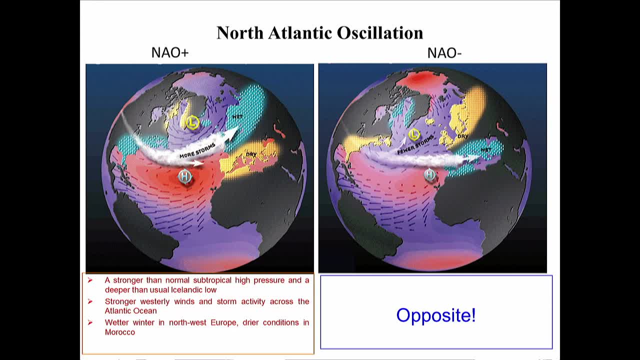 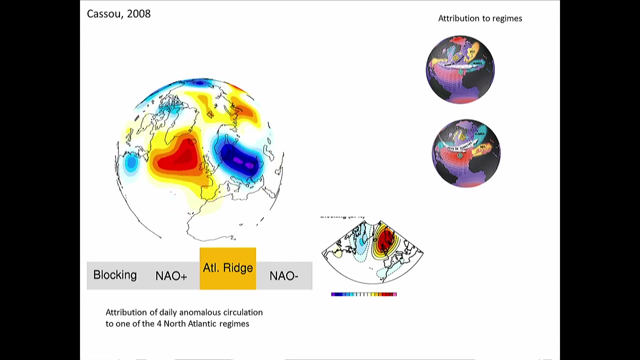 And we have wetter winter in Northeast Europe but drier condition in Morocco And if we are lucky because we need rain in Morocco for agriculture, we end the negative. you know is well correlated with wet condition in Morocco. So last part of my talk, it will be based on 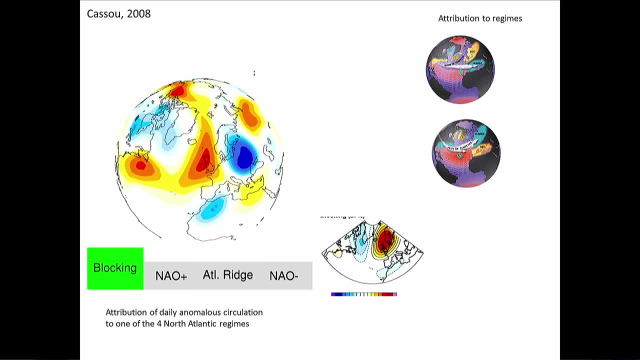 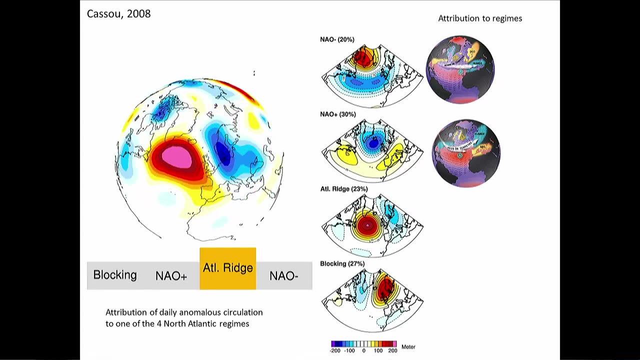 this very precious work of Caso okay, And how it relates to each day, okay, How this work attributes each day, daily animal circulation to one of the fourth regimes, okay. So the idea is: how can we use this connection between days and regimes? first, 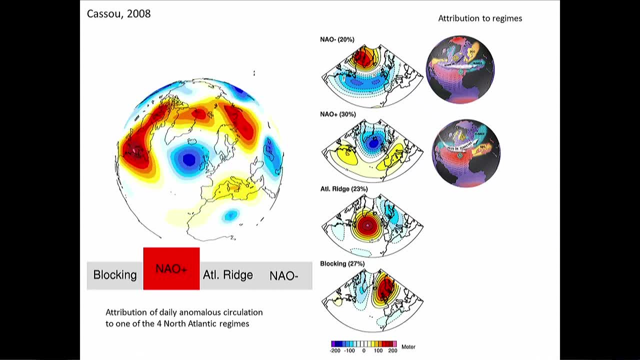 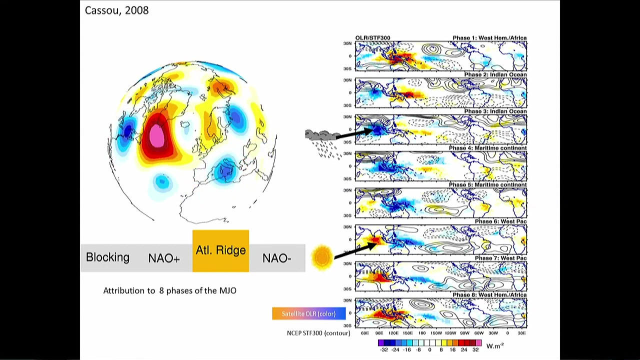 And second, try to understand what control this transition between different regimes. So the positive and negative, you know they are here, as I have mentioned before. So one mechanism that we are interested in in this is this modulating effect of MGO over the occurrence of different regimes. 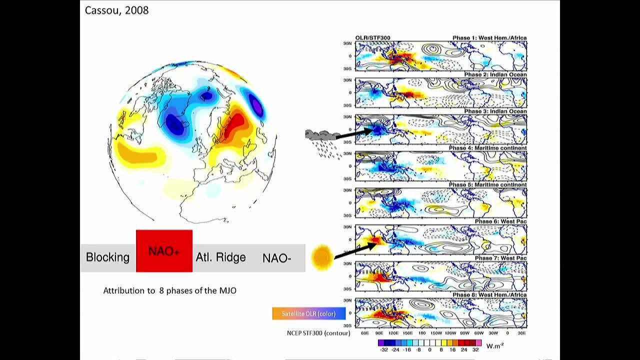 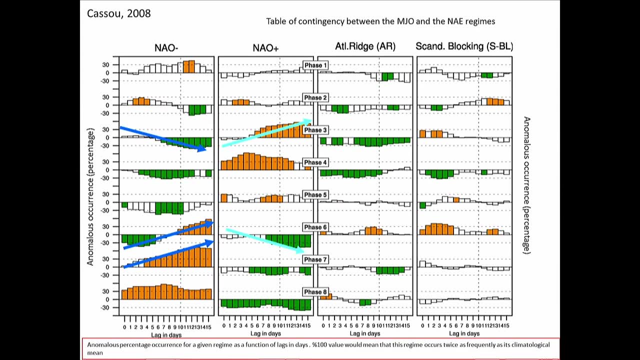 And we are very, and we are very and we are very. at the first time when I have seen this interaction between different regimes and different phases of MGO, I have seen that there is a potential to use this information to relate this connection. 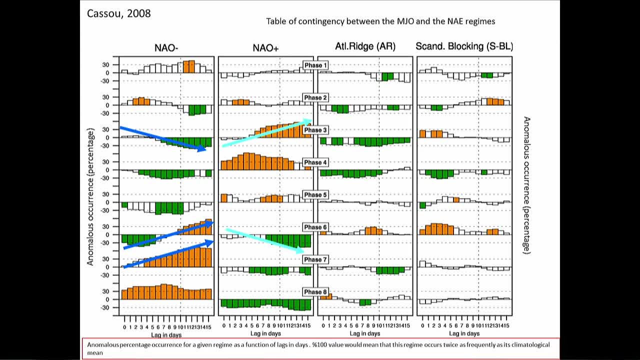 between weather regimes and the MGO phases on the rainfall over Morocco. As we have seen before, the negative phase of MGO is we can have it after 10 days of phase, after phase six- okay, as we see here- And largely over phase seven and phase eight. 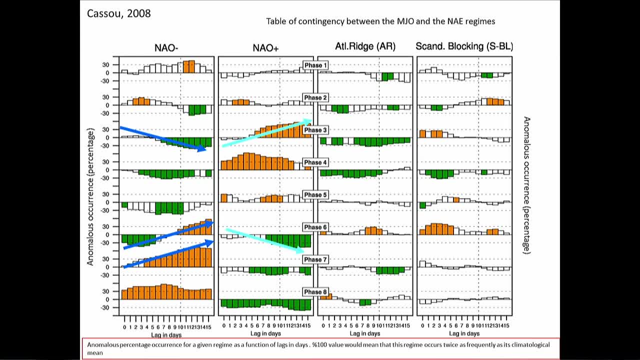 we are in this negative phase of MGO, which is good for us to have this weather condition in perspective, But, on the opposite, the positive phase of MGO. six days after phase three, we have this occurrence of, or forcing of, a positive, negative. 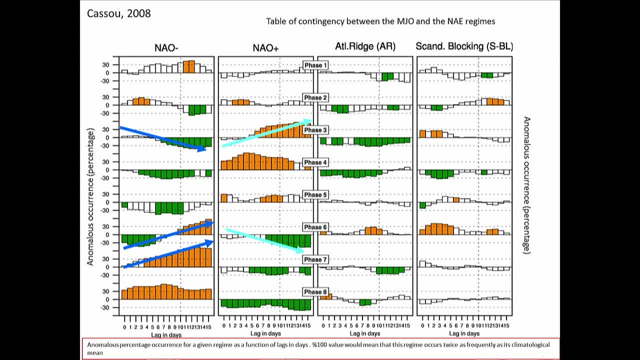 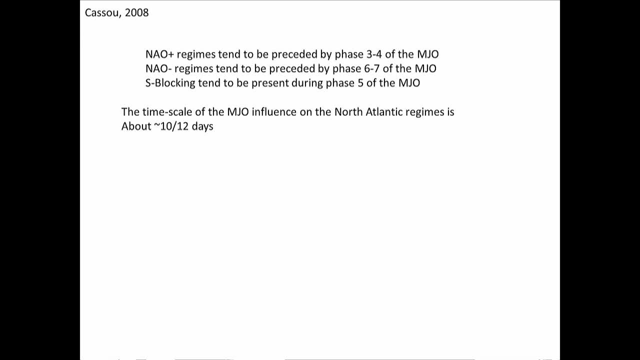 positive oscillation for the North Atlantic. So, according to Christophe Cassoult, generally a positive negative oscillation North Atlantic oscillation regimes tend to be preceded by phase three or four of the MGO. On the other hand, negative oscillation tend to be preceded. 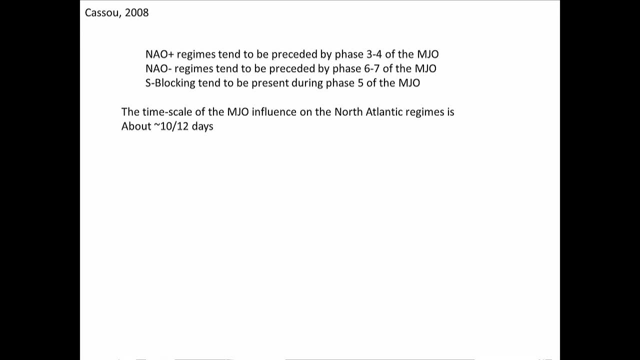 by phase six, seven of the MGO and the Scandinavian blocking tend to be present during phase five of MGO time scale of the MGO influence, which is about in two days. So there is a lagged influence of different phases of MGO on the weather regimes over our region. So, as I mentioned before, 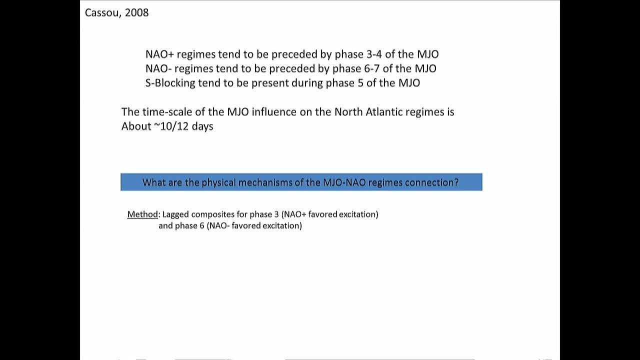 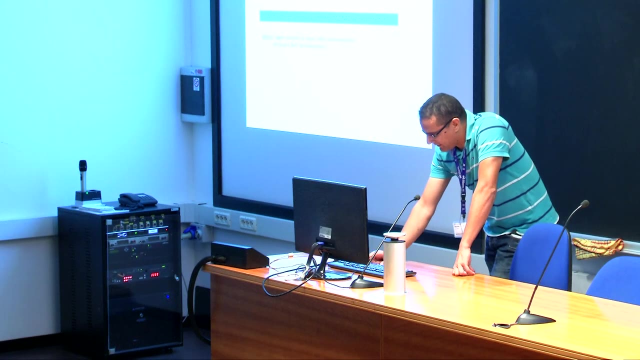 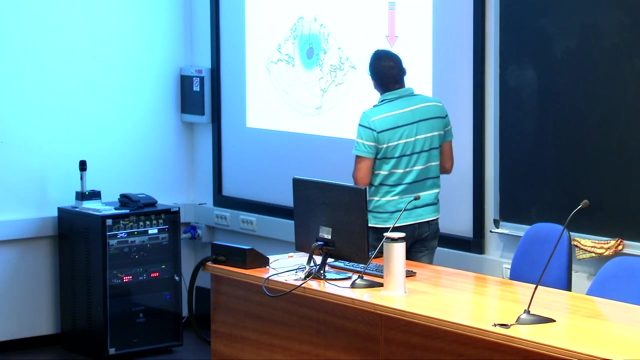 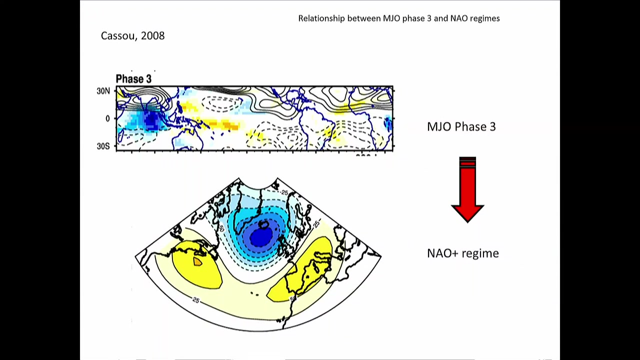 the first part of my talk it will be dedicated to this: physical mechanisms of MGO- North Atlantic Oscillation Regime connections. So as we have just started dealing with this connection, I will present why, if we have phase three in MGO, we're going to end by having positive 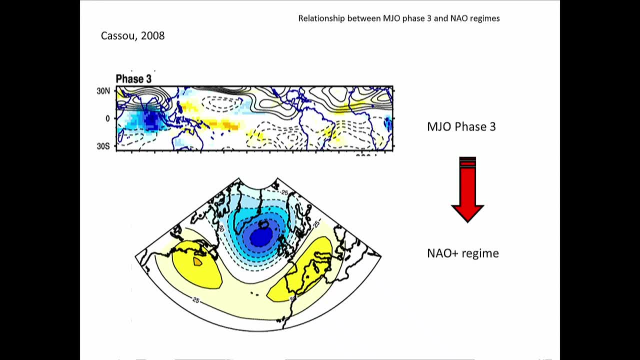 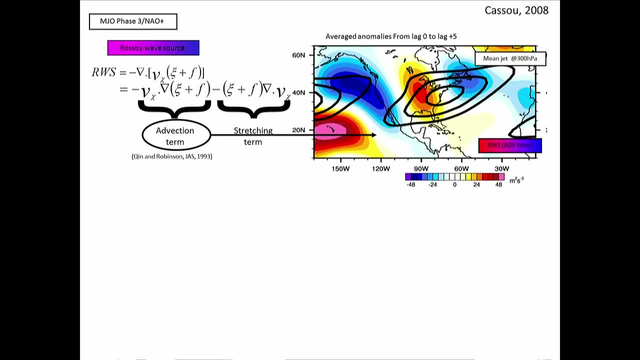 oscillation after 10 days. This is the main observation. So, as we have seen before MGO phase, the MGO oscillation, it will force some Rossby wave excitation. If we are in phase three or phase six we have kind of dipole, We enhance it. for example, 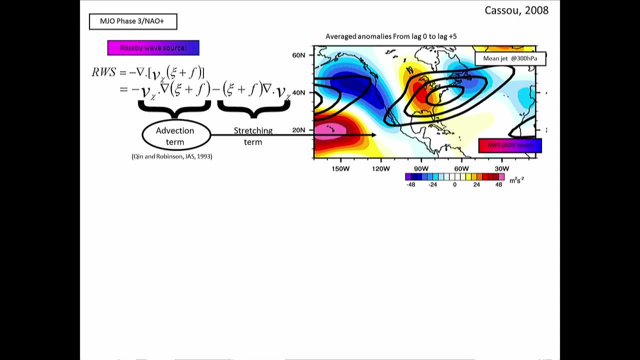 phase three. we have enhanced convection over the Andean Ocean and suppressed convection over the Malian Ocean. We have enhanced convection over the Andean Ocean and suppressed convection over the Malian Ocean. So this dipole will excite some Rossby waves, And if we plot here the Rossby wave source term, 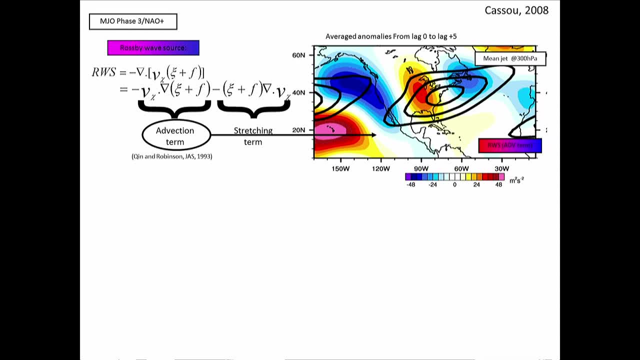 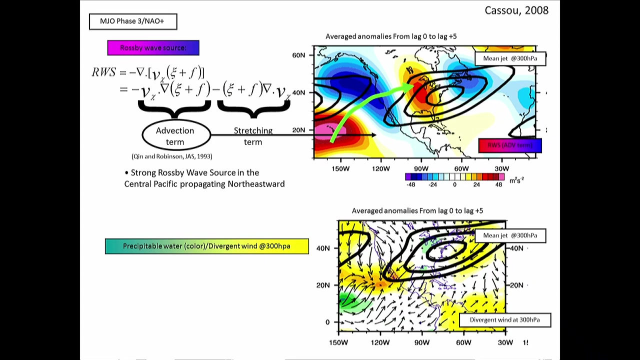 advection term. we see that this dipole has an impact after on the North Atlantic jet stream So strong Rossby wave source in the Central Pacific, it's propagating. It's propagating North Eastward If we try to see what happened in the entrance of the. 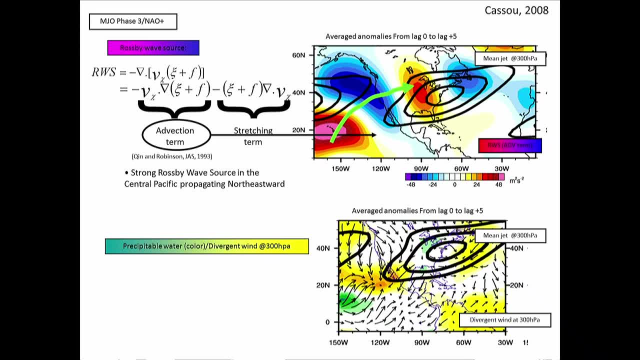 jet stream, of the North Atlantic jet stream. we're going to see that we have related to this Rossby wave source, that we end up by having a strong upper level convergence on the Eastern Pacific and the entrance of the North Atlantic jet And, having also related to this convergence, 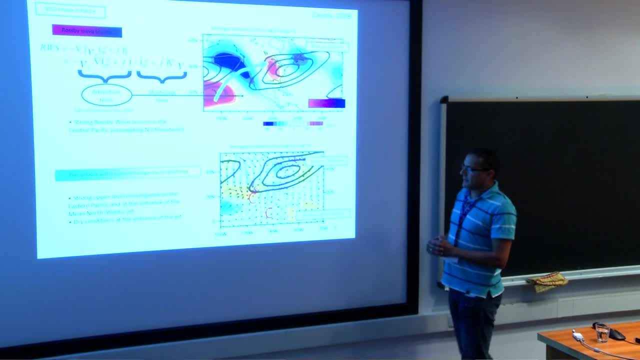 having this gray condition at the entrance of jet. Here in color we plot the precipitable water okay and the arrows show the divergent wind. So here, just at the entrance of the jet stream, we have this strong upper level. 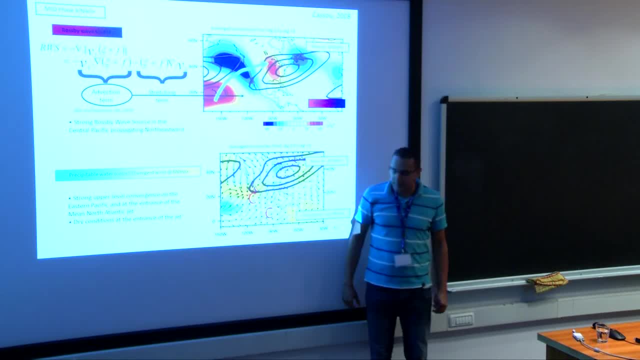 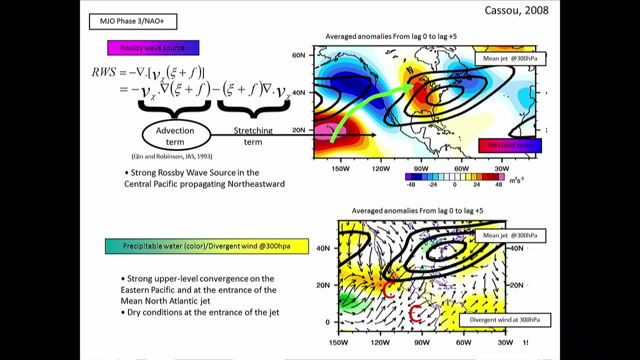 convergence and we have a dry condition at the entrance of jet. It means that our strong tracks they will not have enough supply of humidity at their entrance for the after some days of MGO phase in phase three. But on the other, 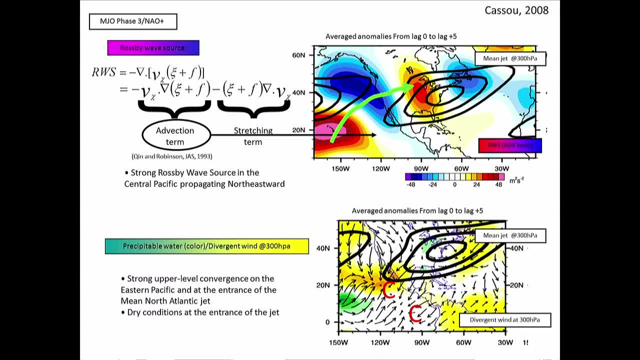 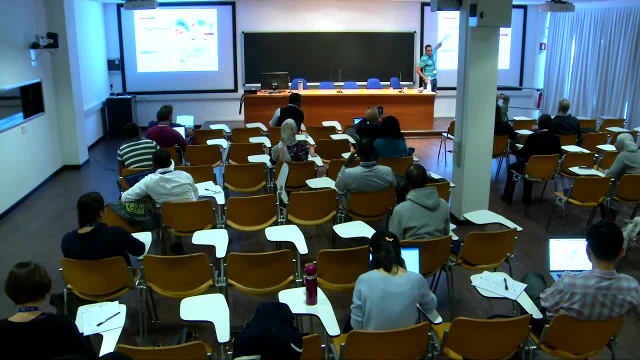 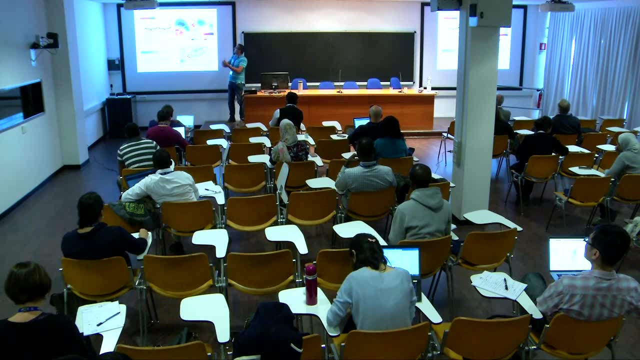 hand Source: okay, The Rossby wave source advection term: Yes, Okay. So we see what happened after five days. okay, after having this dipole of MGO phase over the Indian Ocean and the Maritim continent, What happens after five? 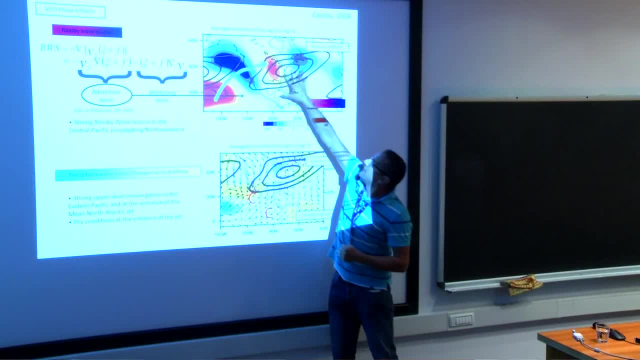 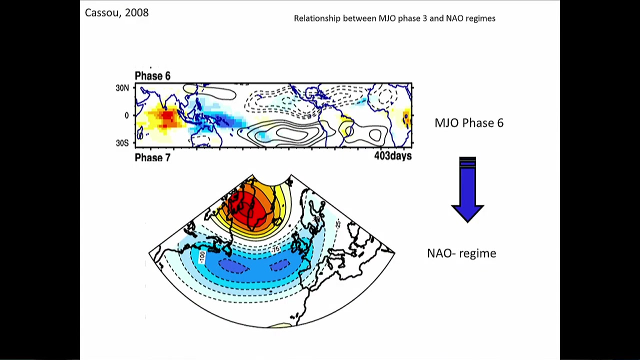 days after zero, five days on this position of the mid, the Atlantic jet, in this convergence zones For the, for the MGO in phase six, and it's forcing of the negative North Atlantic regime, North Atlantic constellation regime, we have some kind of 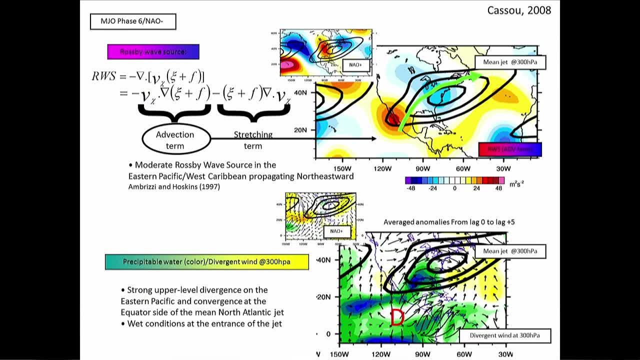 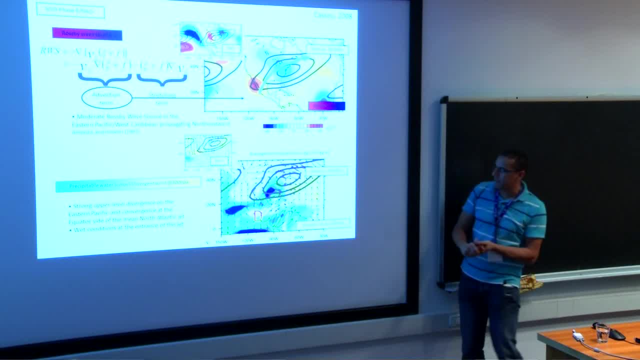 opposite effect. So we plot the same thing here as before. So Rossby, wave source, advection term And what we have now we have. so we have here, like before, precipitation water, Okay, And divergent wind, And here I have this plot, this mid latitude or North Atlantic. 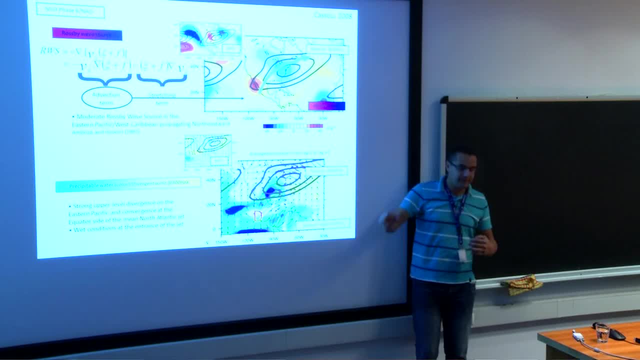 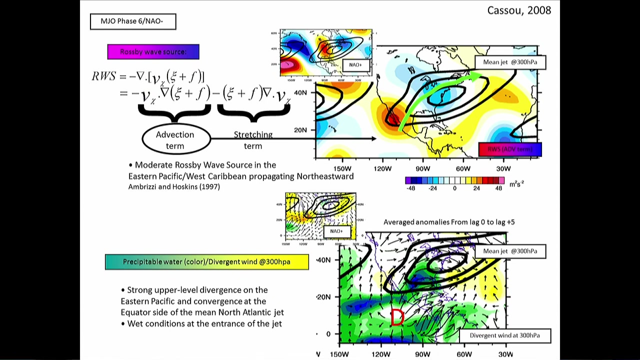 jet. As we can see, we have here the opposite Instead. instead of having this convergence at the entrance and dry conditions, now we have more divergences at upper levels and more supply of moisture, which is good for us because it will. 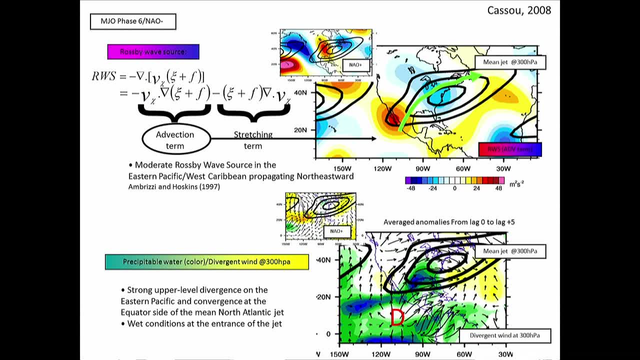 enhance, five days later, more good conditions to how to have this negative well established. This is how I understand, relating to the work of Christof Kassow, this relationship between what happened when we have MGO phase in three and six and what happened in terms of what 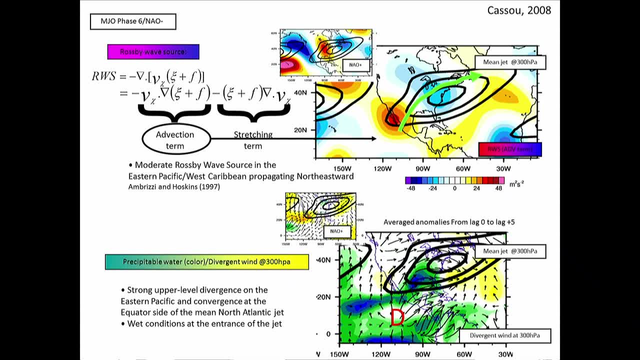 distributional configurations both of water and dynamics over the North Atlantic region, especially at the entrance of the jet. So in a way, this is the bridge with which we have this influence between the tropics and the extratropics. We can see it clearly when plotting these fields. 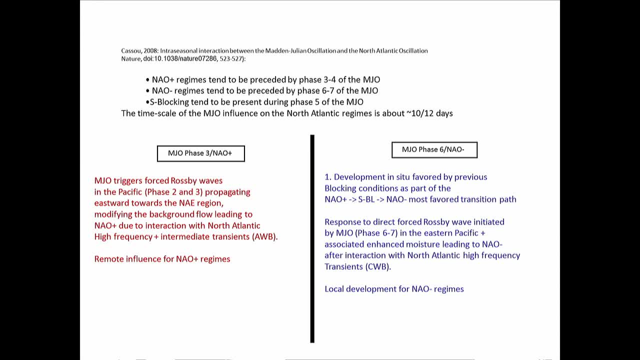 So to summarize the work of CASO, it's kind of overview of the work of CASO. So, as I have said before, MGO: in phase three we trigger fourth drospe waves in the Pacific. With phase two and three we propagate eastward to the north. 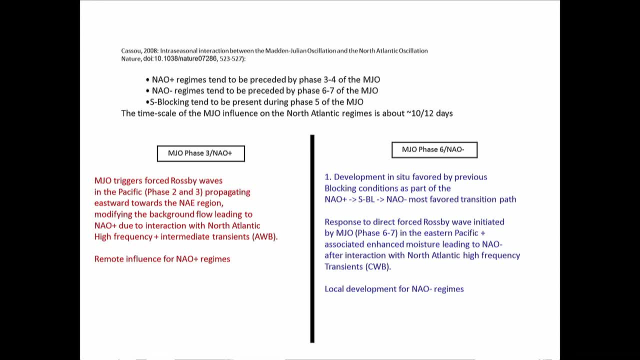 So we have the Atlantic region. okay, modifying the background flow leading to North Atlantic oscillation: positive. due to the interaction with the North Atlantic high frequency plus the intermediate transients, This kind of interaction will have a remote influence for the positives in a way. 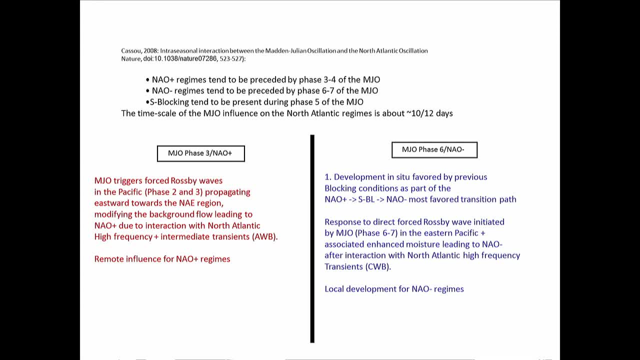 On the other hand, with phase six in the negativities and its relationship with the negative phase of NO, we have a development institute favored by previous blocking conditions as part of this transition that it was mentioned by Laura. So we have kind of preferred transition between the North Atlantic oscillation in positive 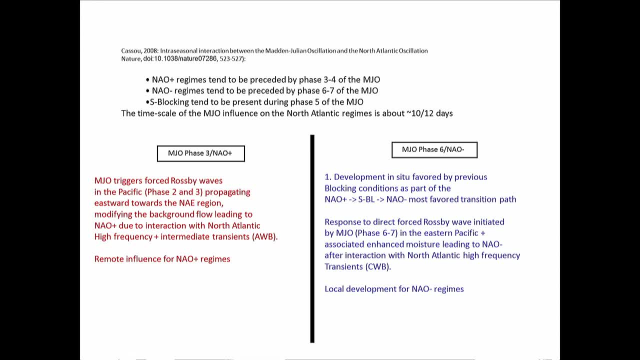 phase. Afterward we have Scandinavian blocking and we end up by having a North Atlantic oscillation in its negative phase. So here we can see that we have this direct forcing of positive oscillation. This is what it was mentioned by Christoph CASO, but here the forcing is not direct. 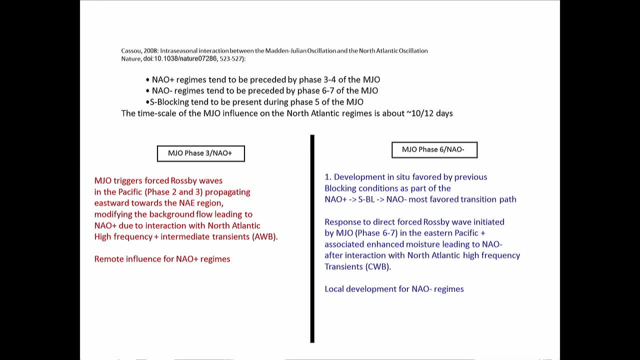 We have this transition by the Scandinavian blocking before having the negative phase of the North Atlantic oscillation. So it's kind of response to direct force of drospe wave, as I have mentioned before with this drospe wave term, Excitation term. 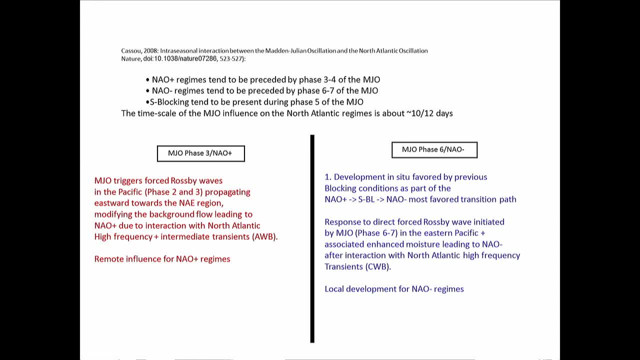 So the response to direct force in drospe wave initiated by MGO in 667 in the Eastern Pacific associated enhanced moisture, leading to this interaction with the North Atlantic high-frequency transient and ending by having what we call cyclonic wave breaking. Is this argued in the paper? 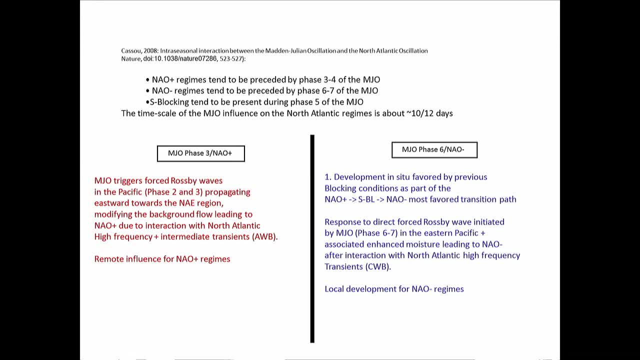 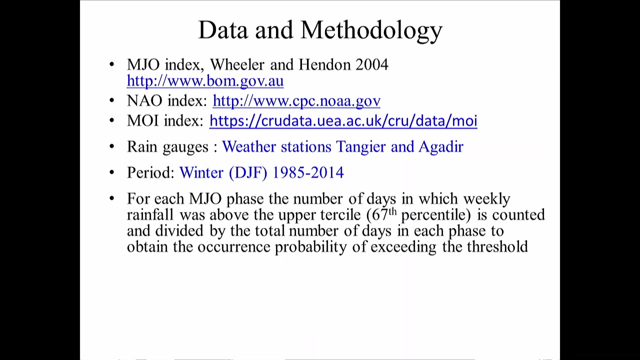 Yes, You added something. It's argued in the paper. Okay, Thank you, Thank you. So, after giving this relationship with MGO in both phases three and seven, and the response over the extra tropics in terms of North Atlantic oscillation, I will show you some results. 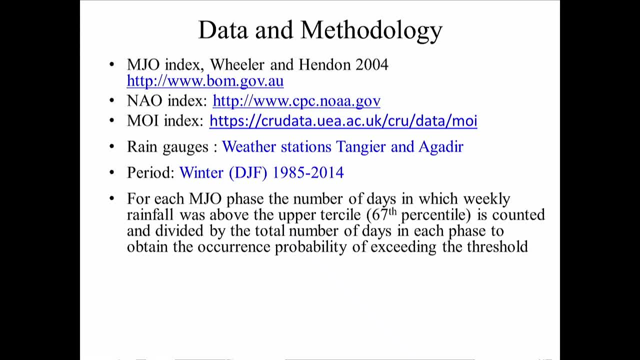 that we have just produced. In fact, we would like to see what happened in terms of precipitation over Morocco. Okay, So, in terms of precipitation over Morocco, in terms of precipitation over Morocco, we have two results related to the MGO oscillation. 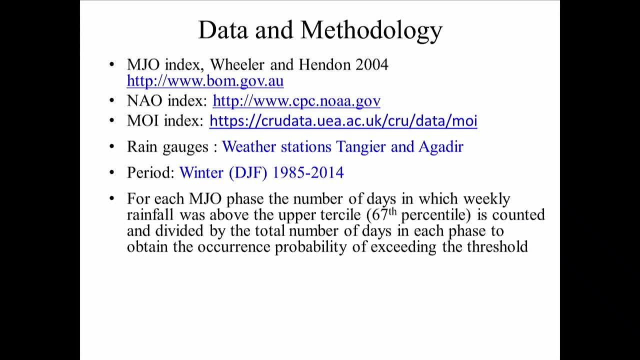 This is the main objective of this first research work. But we are using weather station okay rain gauges from the National Weather Service at two stations, one in the extreme north Tangier and one in the central part of Morocco, near the Atlantic. 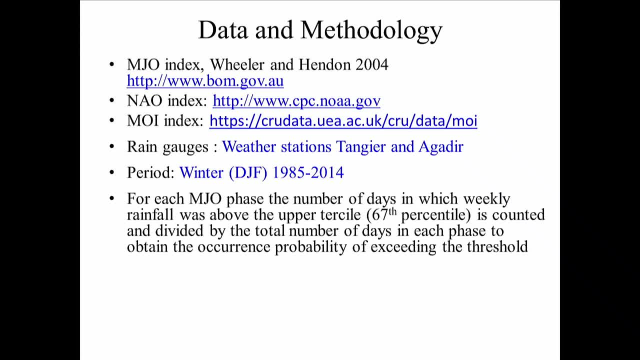 Near the Atlantic, Okay, Near the Atlantic Ocean. So how we do so? we work for DGF. it's our winter season, from 85 to 2014.. And for each how? the methodology is that for each MGO phase, the number of days in 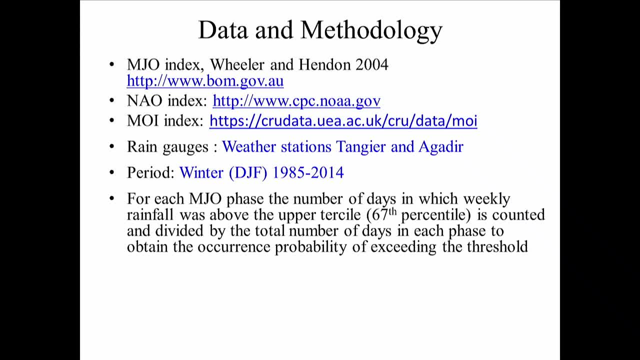 which weekly rainfall was above the upper tercile is counted and divided by the total number of days in which, in each phase, to obtain the occurrence probability of exceeding to the threshold. So the occurrence probability that I will show later is calculated following this method. 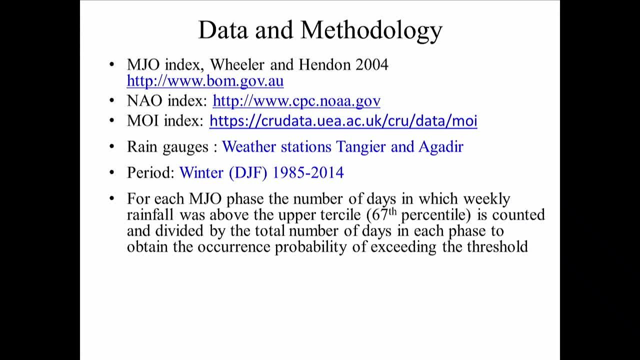 So each phase we count the number of days in which weekly rainfall was above the upper tercile. So we have chosen this upper tercile because it has been mentioned before in other works. That is a good threshold for trying to find this oscillation, this relationship between. 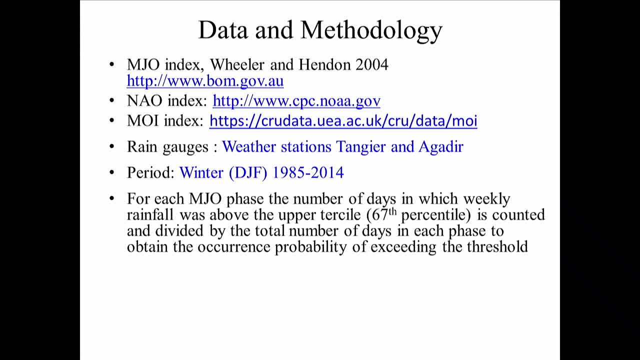 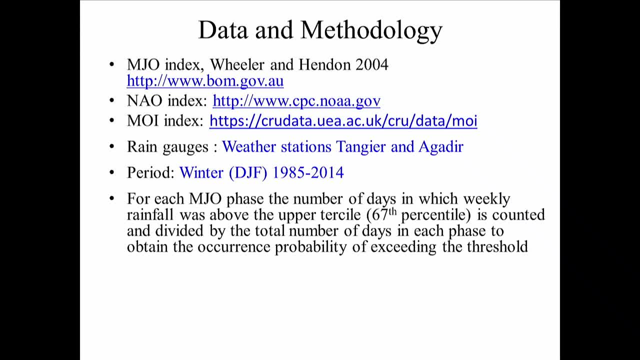 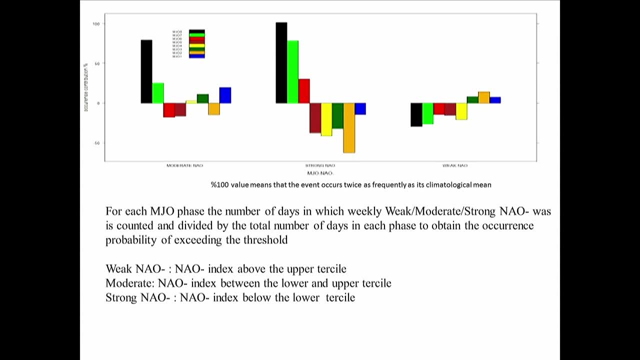 It is also a running mean. So a running, seven-day running mean. Here is the outcome of the first statistics that we have done. Okay, So here for each phase of MGU, the number of days in which weak- weekly weak, moderate, strong. 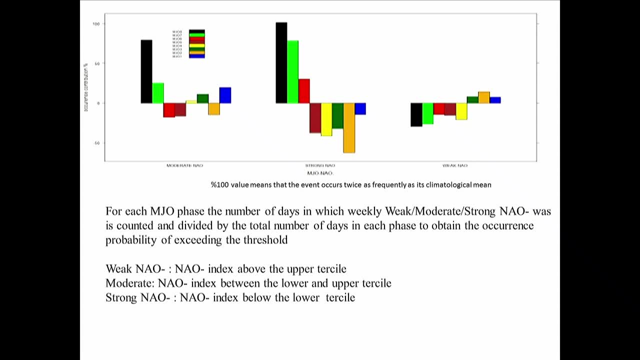 in our negative is counted and is divided by the total number of days in each phase to obtain the occurrence probability of exceeding the threshold. The same as before for precipitation, we do it for North Atlantic oscillation in its negative phase. So the weak negative phase is where our index is above the upper tersile. 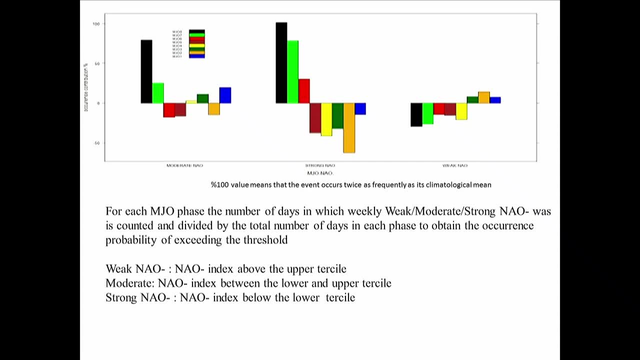 Moderate is between the lower and upper tersile And the strong one is when the negative NO index is below the lower tersile. So as you see, here for MGU NO relationship with when we have a strong NO. we see clearly that. 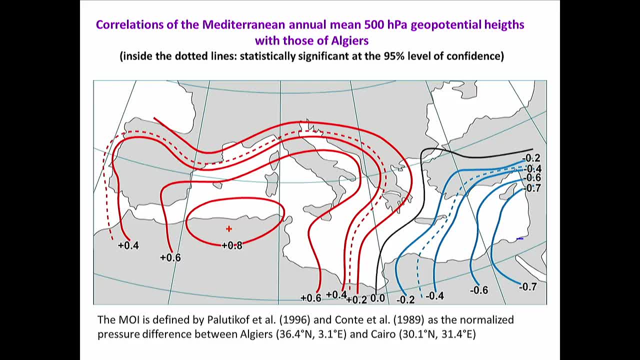 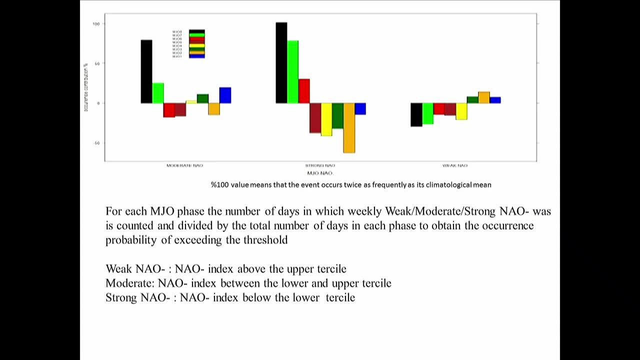 Here I have in blue I have phase 1, and in red is phase 8.. So here I go from phase 1 to phase 8.. So for strong NO- the event where I have a strong NO- we see that the occurrence of strong NO happens with a grid function. 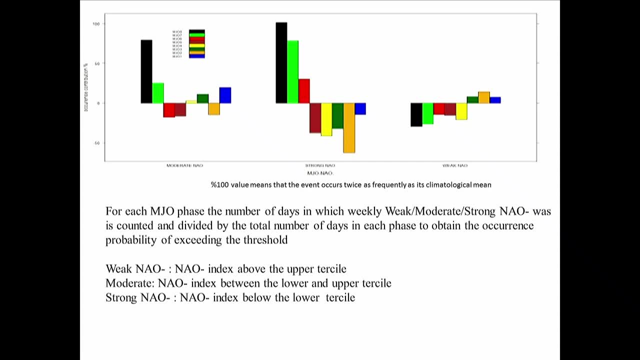 And this is the frequency when we have 7,, 6,, 7,, 8 phases of MGU. So the impact is more clear. when picking the strong NO negative events, We have the same thing for the moderate NO: It's in its negative phase. 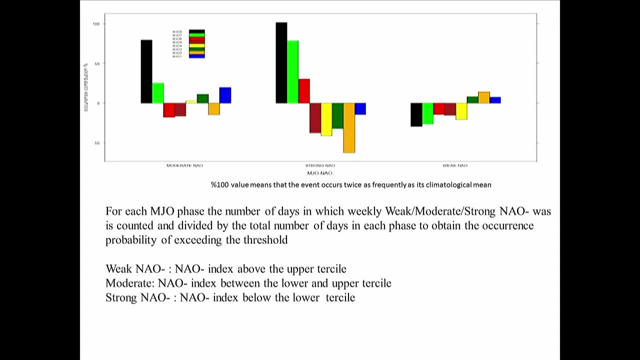 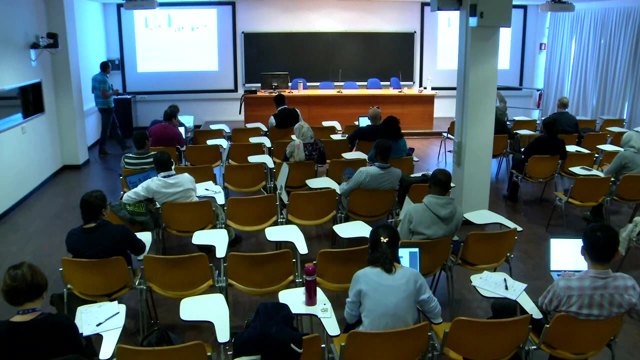 We have phase 6,, phase 7, and phase 8, which are the dominant and the negative. So we have a dominant here for this moderate NO occurrence. So it's the same, Sorry, sorry. So in Marx the type of expression was more or less negative. 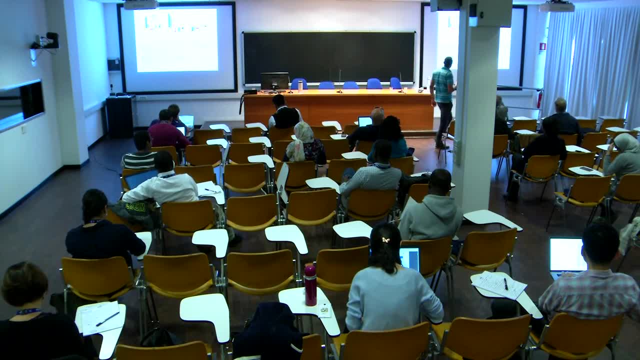 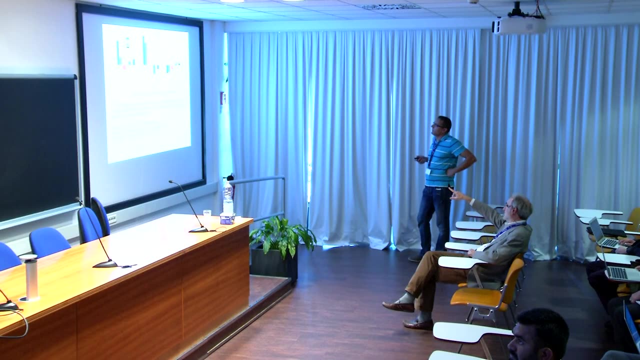 So if we focus, say, on the central histogram, which is for the strong, negative, NO, am I right? Yes, So the black bar is 1.. 1,, 2,, 3,, and then you go up to 8,, east to blue. 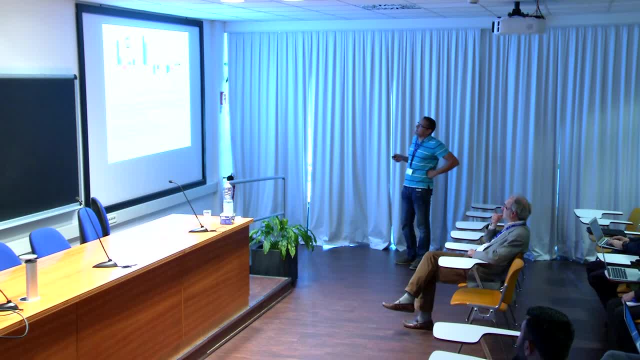 Yes. So here it means that with this frequency or this occurrence contribution, it means that in phase 8, strong NO, it will occur twice as frequently as its climatological mean. with this 100%, Okay, With 100%. 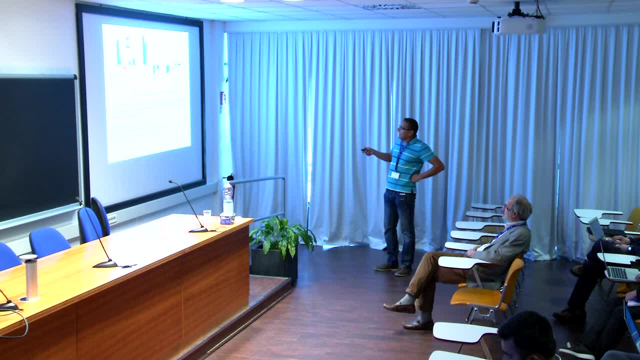 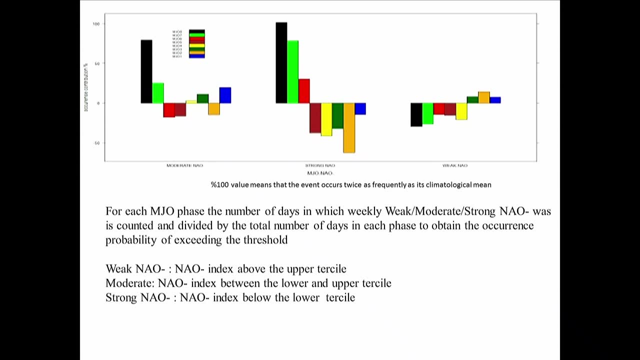 It means that in phase 8, there is a chance to have strong NO in negative phase twice as frequently as its climatological mean. Oh, okay, Sorry. So black is 8.. Black is 8.. Green is 7.. 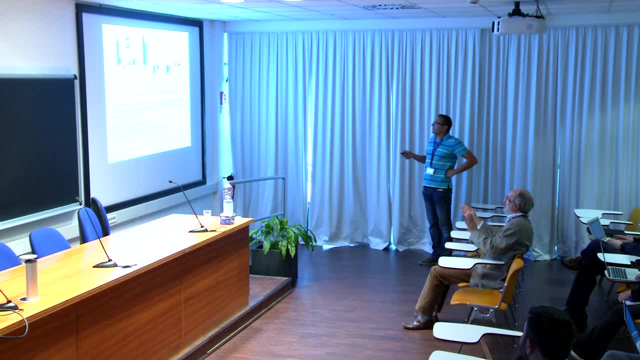 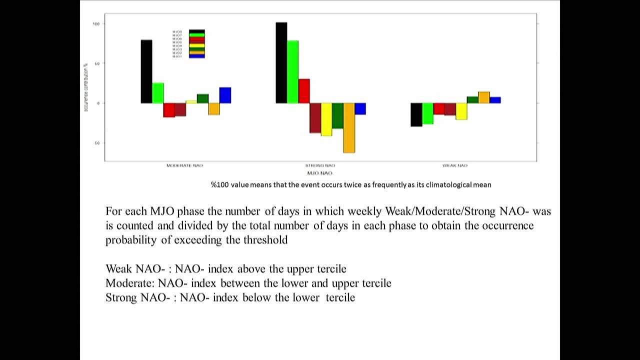 Oh, okay, Yeah, no, Because yeah, that's important. So black is 8,, green is 7, and red is 6.. And then okay, And the others 1.. So we see that for 6,, 7,, 8,. 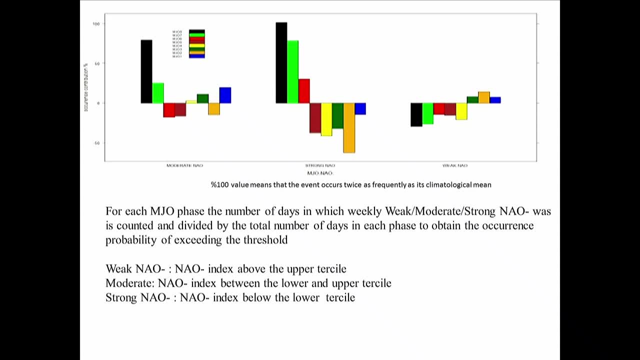 we have an increase of the occurrence probability of the negative phase of NO, especially for strong events. So it is in line with what has been found by Christophe and by Hai. Yeah, yeah, No, it was simply deodorant- from 8 to 1.. 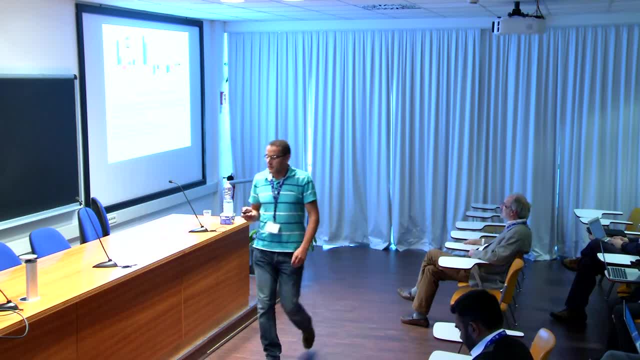 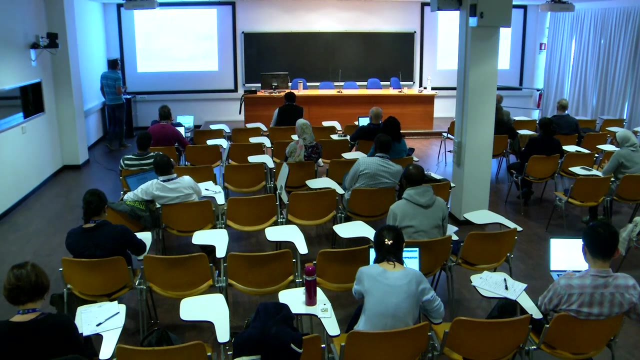 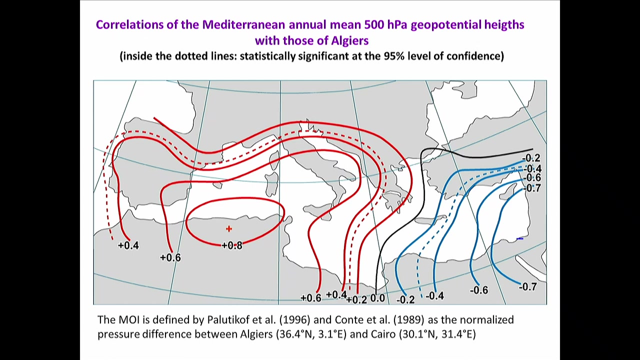 I thought you need to So it is clear for everybody here. So we have also been interested to see what happened in terms of occurrence for the Mediterranean Oscillation Index. Okay, We have kind of Mediterranean Oscillation Index which gives a measure of what happened over the Mediterranean. 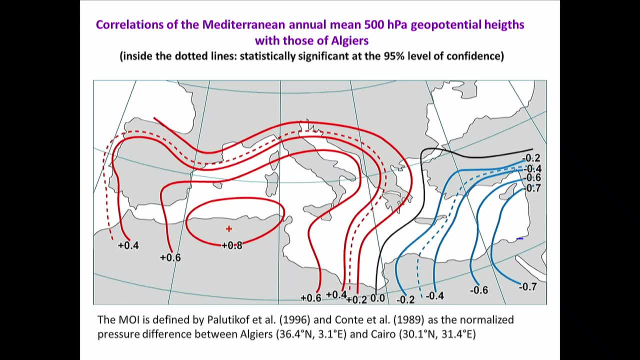 Okay In terms of oscillation. there is kind of CISO also in terms of pressure between Algiers here, okay, and Cairo here. So when we have negative here we have low pressure here compared to this location in Cairo. we are in this Mediterranean Oscillation in its negative phase. 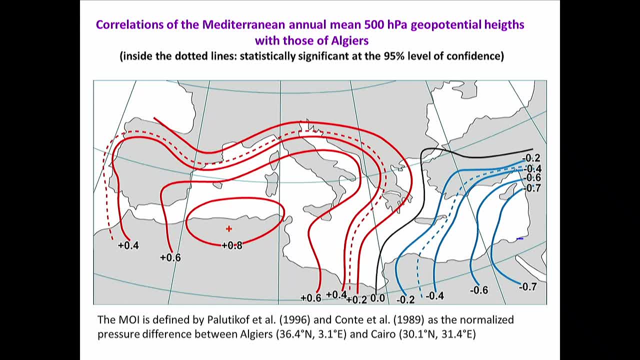 So Mediterranean Oscillation is in negative phase. It's something that is good also for Morocco, because we will have storm or low pressure systems that will interest the north part of Morocco. So we have also tried to find if there is any relationship between the occurrence of this Mediterranean Oscillation. 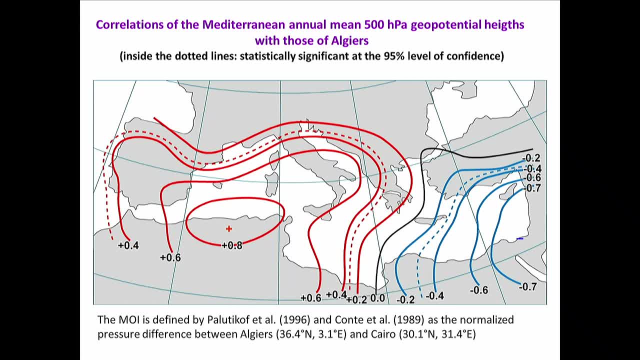 and the different phases of MGO. Okay, See, here it's just to show that there is a CISO. so between the two regions. okay, Here we correlate Algiers geopotential height at 500,. okay with other points. 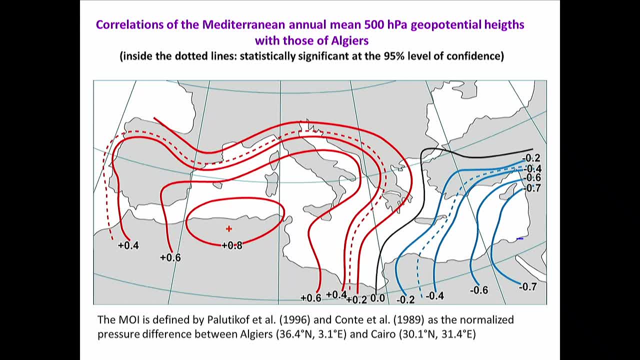 It's just a correlation, okay, between this point with other points And we see that we have this dipole. okay, It means that we have some kind of oscillation. Mediterranean Oscillation is based. It's based on the fact that what happened here in terms of pressure, 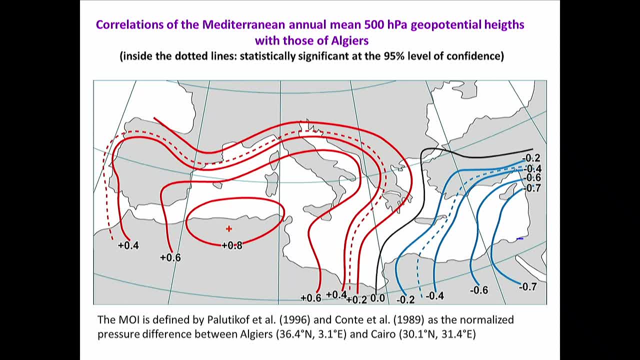 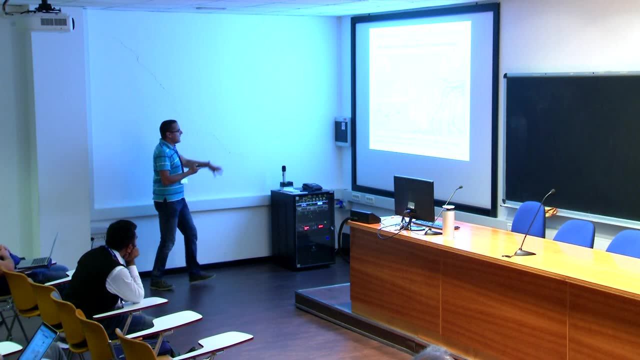 it may be anti-correlated with what happened here over Cairo. So we have this Mediterranean Oscillation index. It's a measure of how far, in terms of pressure, are from Algiers to Cairo. So here, when you have a negative phase of MGOs, 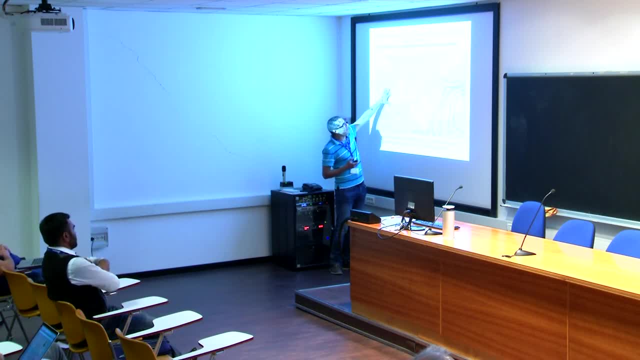 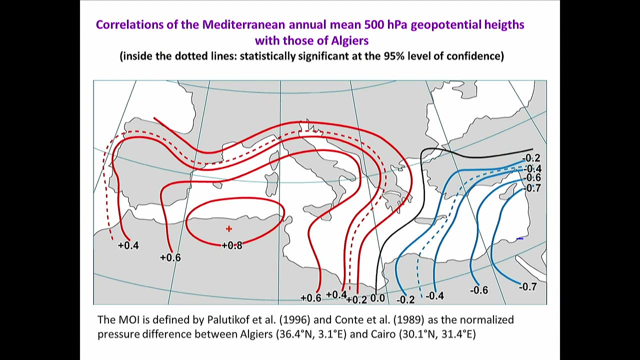 it means that we have here a low pressure system, So high frequency of low pressure systems here We'll have a high pressure system, Cyclonic here and anti-cyclonic here. It means when we have here a cyclonic, it means that we have a chance to have precipitation over Morocco. 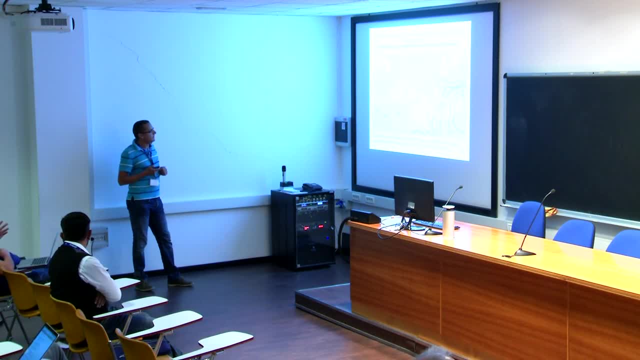 So there is a kind In the case when we have a low pressure system here, okay, and when we have here a cyclonic anomalies, and we will have here anti-cyclonic anomalies, it means that we have Mediterranean Oscillation in its negative phase. 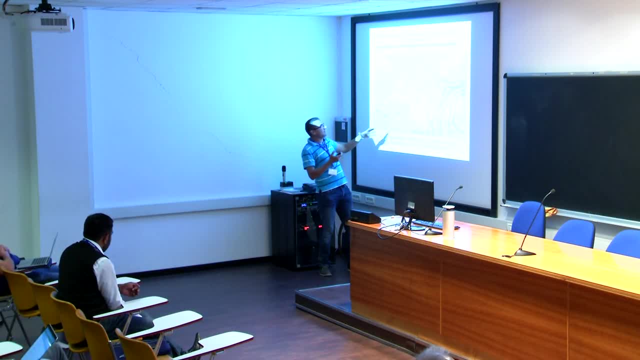 So this correlation, it just show that all this region doesn't behave as the same as this one. So we have some kind of oscillation that we may measure by having the normalized difference pressure between this spot, which is Algiers, and this spot, which is Cairo. 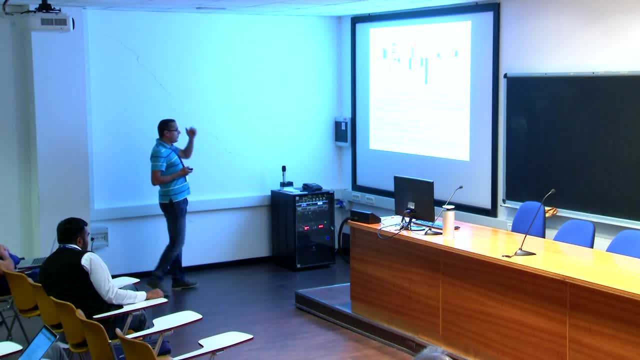 So here we have the same, so the same methodology as before. So we can see here something very special for the strong Mediterranean Oscillation events in negative events. So we see that the blocking or not the blocking, the phase in phase six, okay. 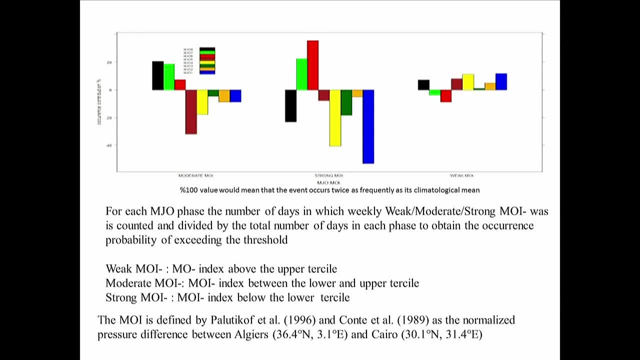 we have high pressure, So we have a high occurrence of strong Mediterranean Oscillation negative- okay compared to the other phases. In fact, what happened here? it's the same. the behavior here is the same of what happened for what has been found by CASO. 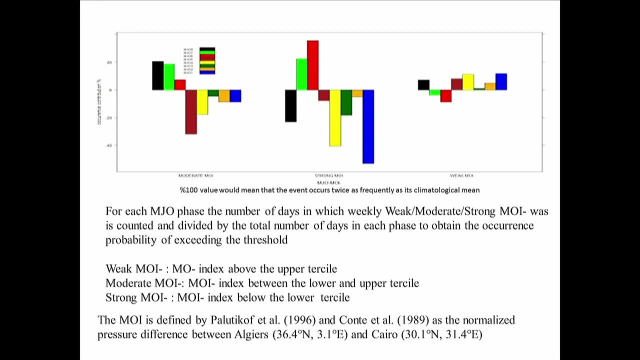 when we see the blocking regime. So in phase six we have high pressure, We have a high frequency of blocking regimes And here, in phase six, we have high frequency probability of having a strong Mediterranean Oscillation. This is the message that we can have from this plot. 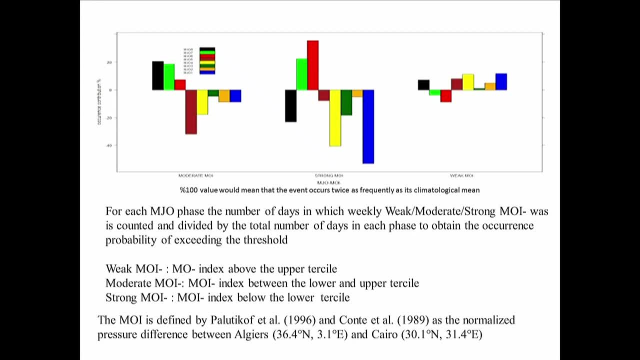 And so of course we have very here reduced occurrence of strong Mediterranean Oscillation in phase one. So this is kind of So, this is kind of So, this is kind of of relationship that we can have also when we try to see this relationship. 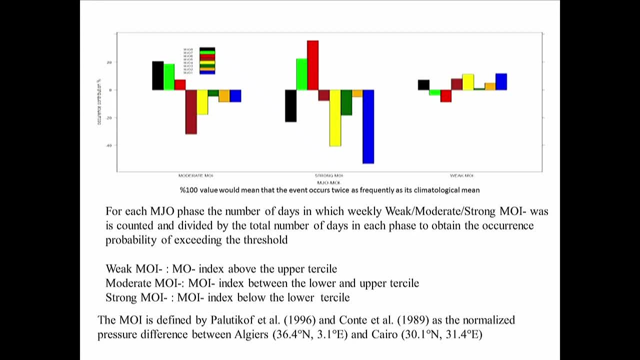 with the MGO and the Mediterranean oscillation. My explanation why we have this strong occurrence or high frequency of Mediterranean oscillation in its negative phase when we have this phase 6, is it in fact related to the same finding as Christophe Casseau? we have more chance to have. 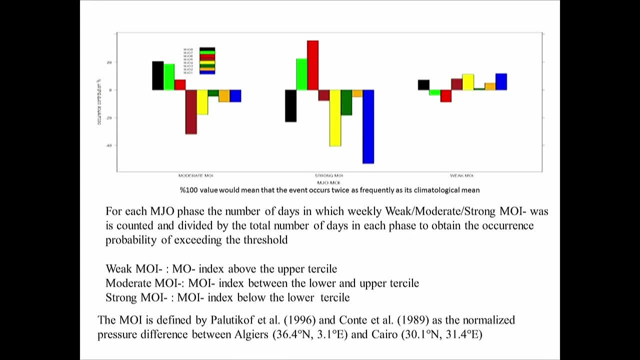 negative Mediterranean oscillation with this transition between, with its transition to the blocking regimes. There is something very important here, in fact, in Morocco, during my experience as forecaster. there is something very important here, in fact, in Morocco, during my experience as forecaster. 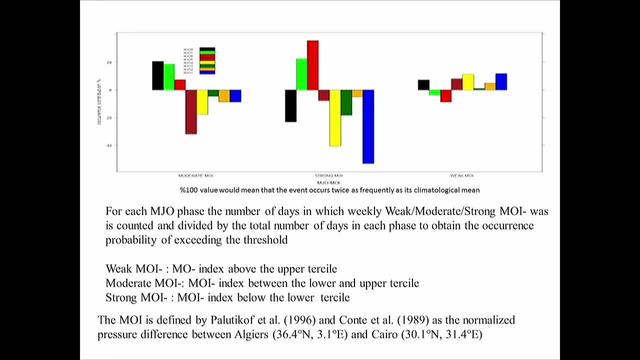 I have seen that generally wet conditions over Morocco they happen, especially when I have this transition between the Atlantic Ridge and the Scandinavian blocking system. It's something that maybe I will one day present some results on this transition, preferred transition between the Atlantic and the blocking. 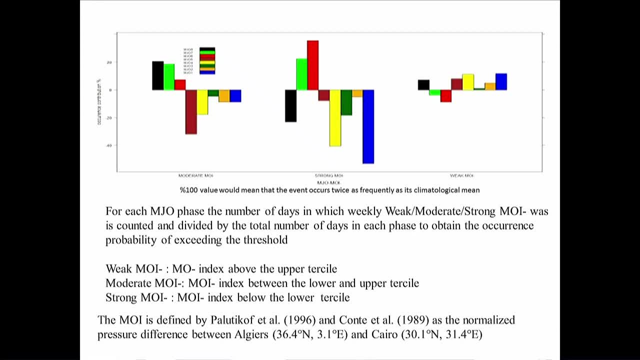 not preferred, but something that happened to not preferred but something that happened to. it's related to precipitation over Morocco. So we will have this chance to have this transition between the Atlantic Ridge and the blocking. there is a chance of having wet conditions over Morocco. 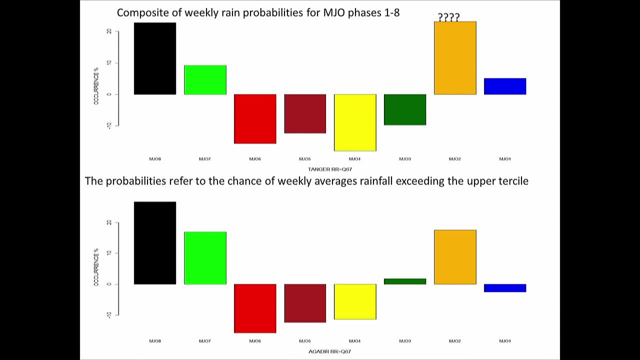 Here- this is the main plot of our first result- is to see the. Here- this is the main plot of our first result- is to see the. how rain fall in Tangier, so the extreme north of Morocco. so measured from rain gauges from 1985 to 2014. 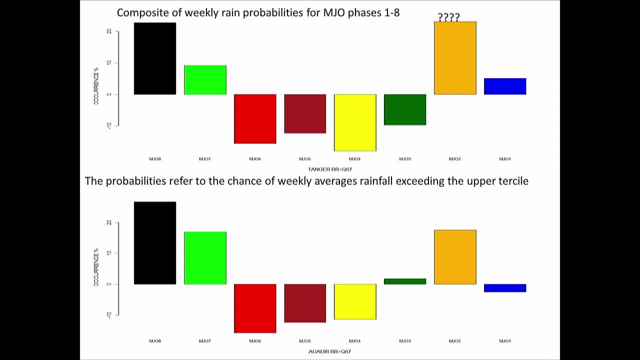 how this precipitation relates to the MGU in different phases. ok, We see here, phase In, phase eight, The occurrence probability it increased to have a precipitation that exceeds the upper profile. Is it good, Is it fine? Because we have this relationship between negative, you know, and phase 7 and 8.. 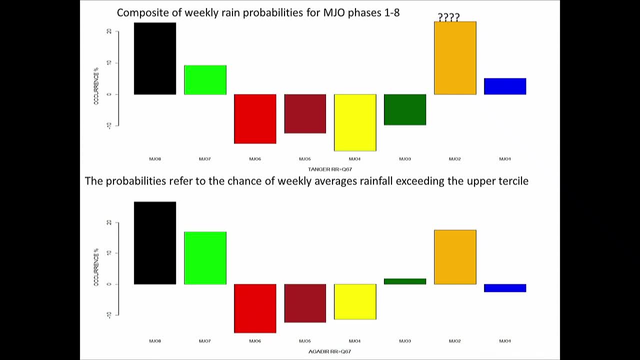 So we can find the explanation why we have this increase between when we have this phase 7 and 8. Why we have this increase of the occurrence of precipitation exceeding this upper profile. But for phase 2, up to now, we don't have any explanation. 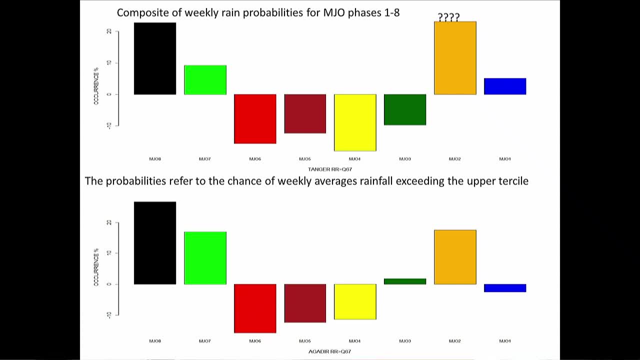 The same thing for this second station. we have the same signal, So over the same period. we in a very distant location, so I get it. it's in the central part of Morocco, near the Atlantic Ocean. so we have the same signal in phase 2.. 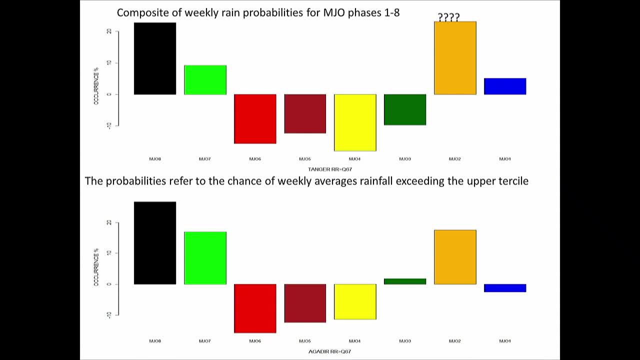 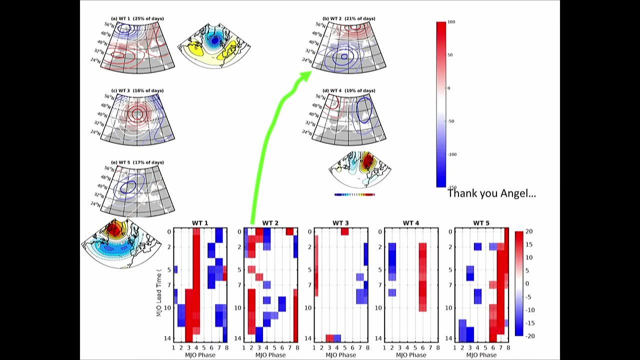 So there may be something behind this preferred occurrence of precipitation exceeding the upper profile in phase 2.. And here I will say thank you to Angel, Because before coming to you I didn't say thank you to Angel. I didn't say thank you to Angel. 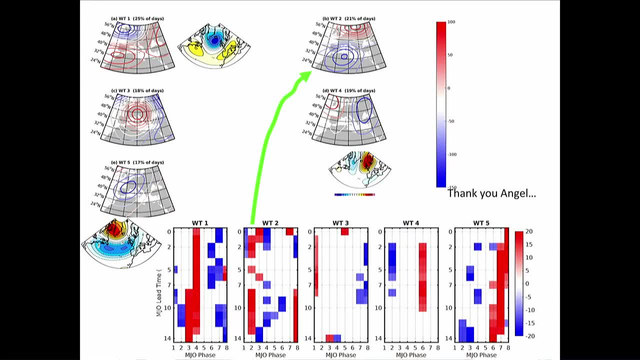 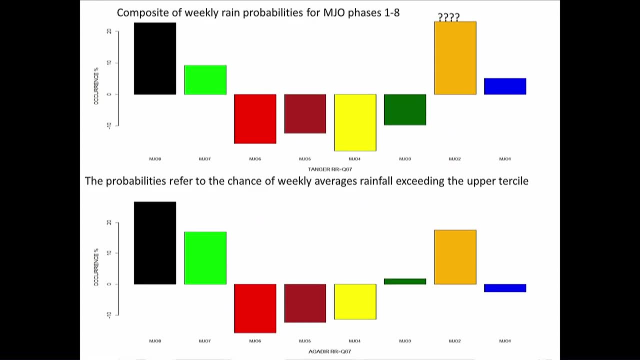 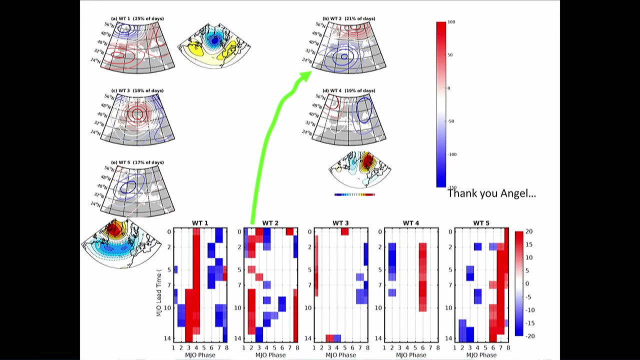 I didn't say any explanation why we have this increase of occurrence, of probability, occurrence in phase 2.. Because I don't have a negative in order to explain why I have this increase. In fact, the idea is that over our region, over the Oro Mediterranean region, 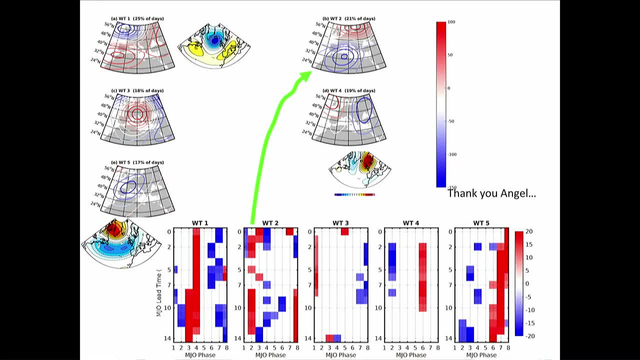 the four regions are not enough to explain what happened In terms of weather types. That's why, using the precious tool of Angel, I have produced another extra weather type, which is what's missing for our region of interest. So here we can see the NO in its negative phase. 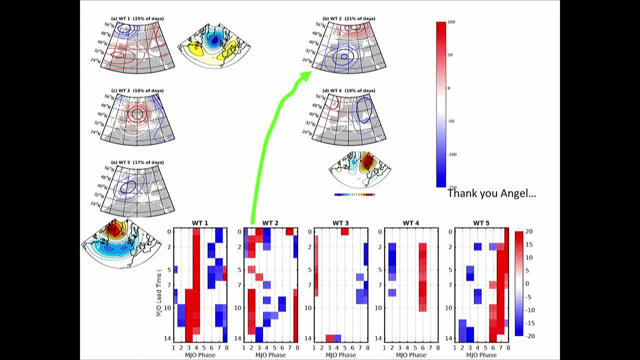 is weather type 5. We can see in weather type 4, the blocking, the Scandinavian blocking. so it's the same. Here they are similar, these two plots, two maps. Here we have kind of similarity between a positive in a U and the weather type number 1.. 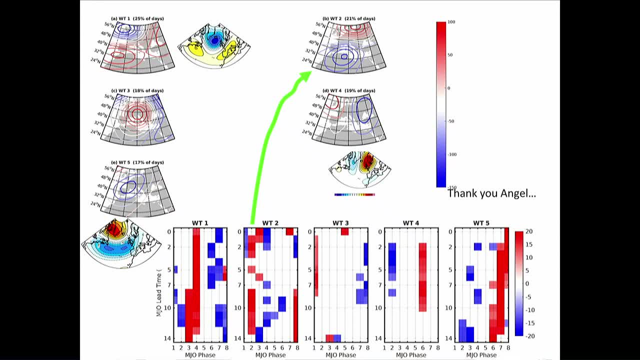 And here I have two patterns or two weather types that are different. Okay, this one, The weather type 2, is it can explain something for me for this relationship between phase 2 and what happens in terms of precipitation. Here also, I plotted the same with the same tool of Angel. 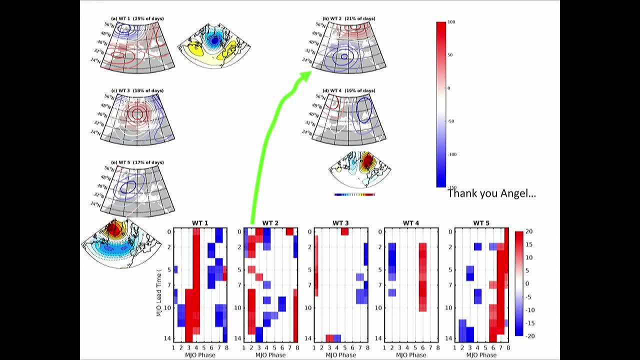 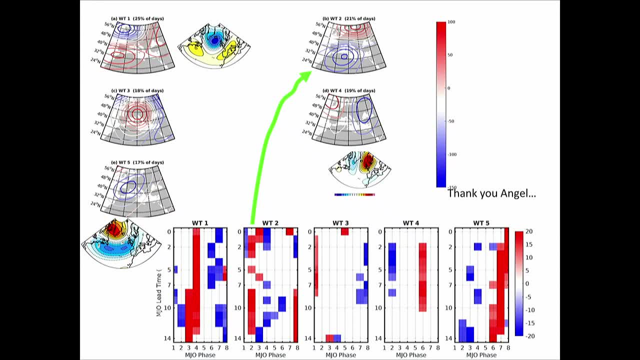 As you see, in phase 6,, 7,, 8, we have an increase of the probability occurrence probability of weather type 5, which is close to negative in a U. So it supports, it does support the finding that we have before. 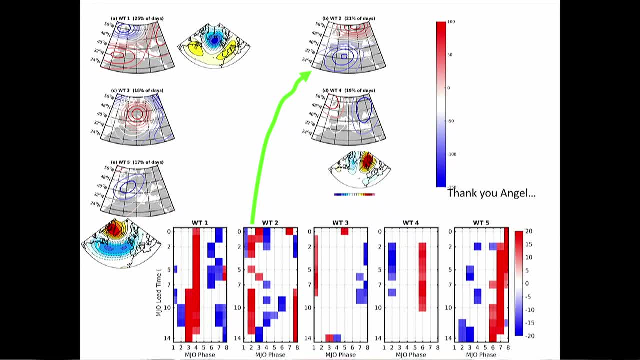 In phase. in phase 7,, 6,, 7,, 8, we have more frequency of negative phase of in a U. This is the first result, So it supports all the finding of Castle Christophe A and high. 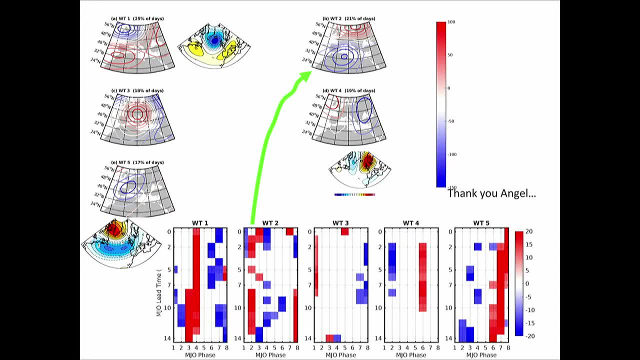 This is the first result. The second one here, when MGO is in its phase 3 and 4, we increase the probability of occurrence of weather type 2, of weather type sorry 1,, which is similar to the positive North Atlantic oscillation. 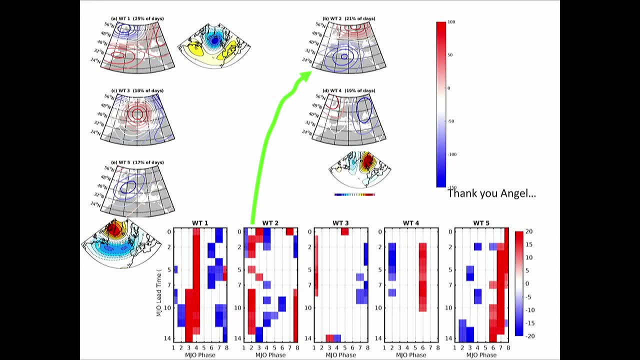 So it is in line with the finding that of Christophe and high. So it's fine, Here there is something new. So in phase 2, we see that this weather type is more frequent compared to the others. 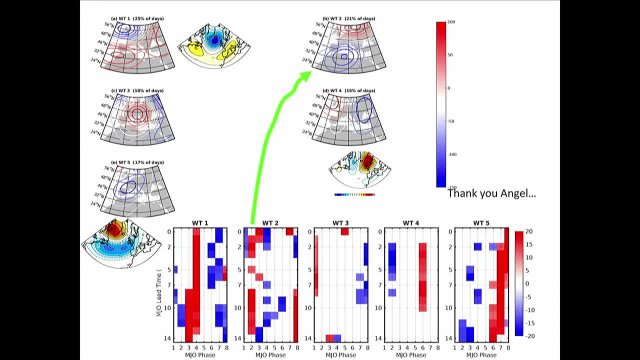 And also it is MGO is in its phase 3 and 4.. MGO is in its phase 3 and 4.. MGO is in its phase 3 and 4.. So it's favorable. It's a weather type that is good for having a precipitation over Morocco. 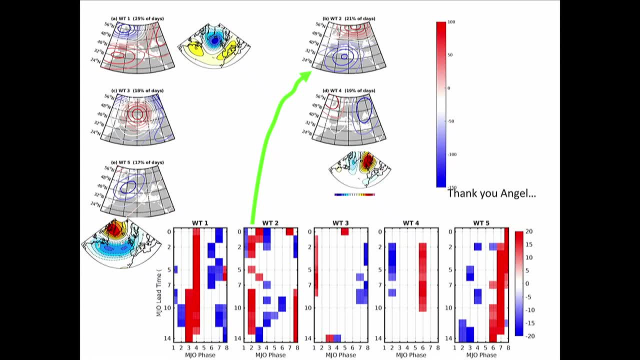 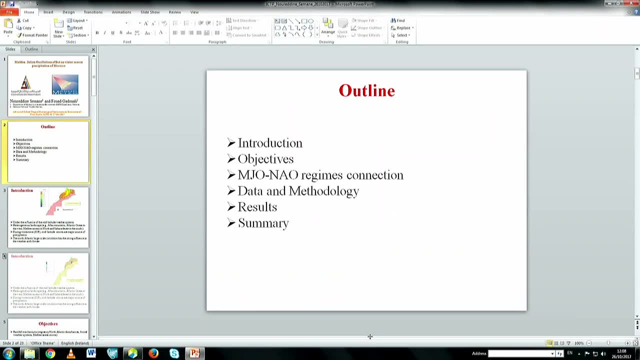 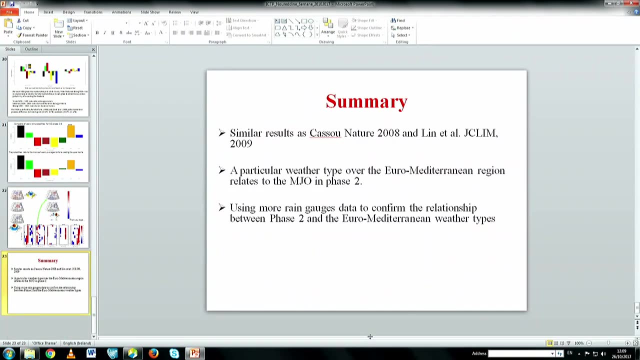 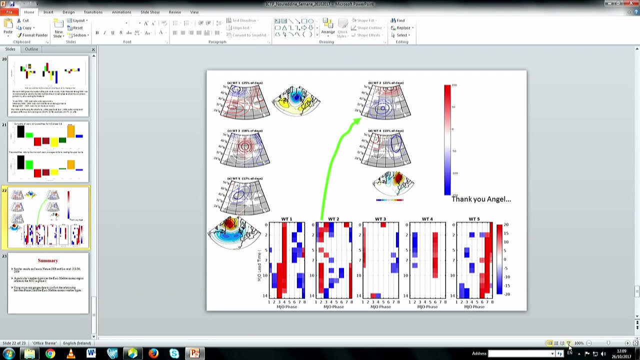 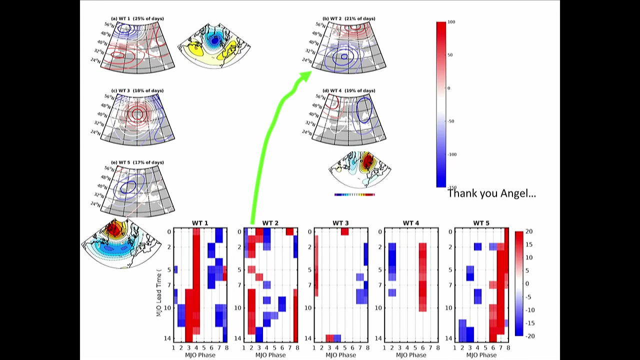 because we have here a negative anomalies of geopotential height at 500 HPA. So sorry, Let's make it back. Okay, How do I put it here? So we have now found a relationship between these extreme events- not extreme, but for high amount of rainfall observed over Tangiers and Agadir. 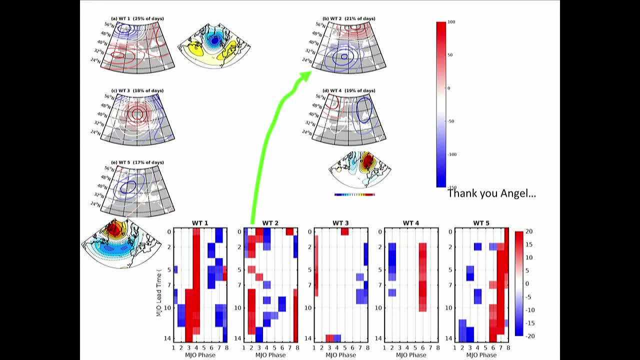 that are related to a weather type which was not present in the classical classification of weather types over the North Atlantic. In the North Atlantic region we found this with this new weather type which is more favorable to have a wetter condition over Morocco when we have phase 2..